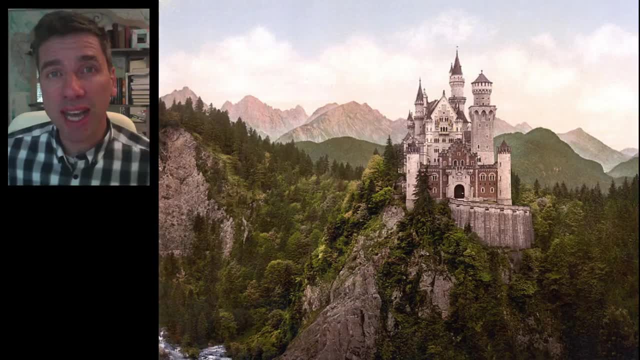 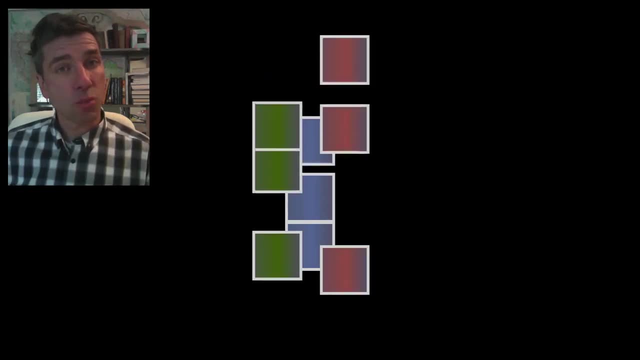 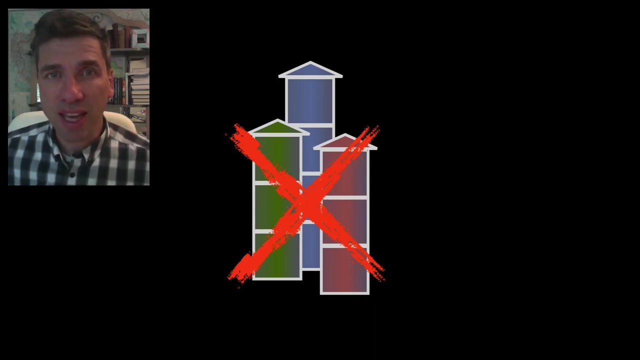 He tells you that he wants you to build him a magical castle. He's got enough money to pay for ten stories. So this is one possibility. But he says no, you can't do that because two of the towers are the same height. 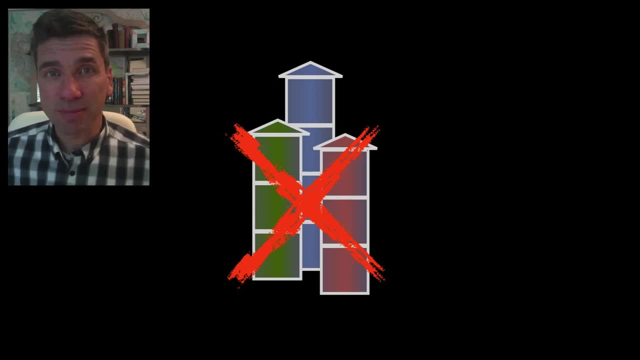 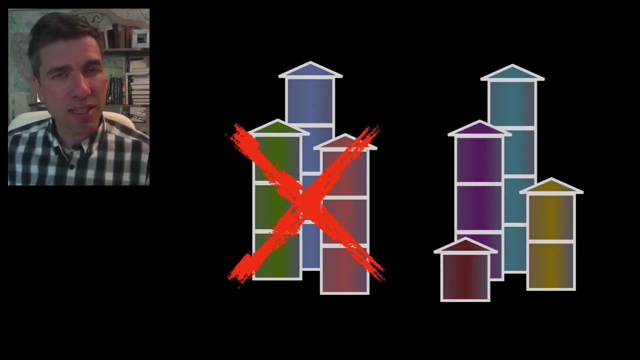 He wants all of the towers to be different heights. He is eccentric. Let's see, does this work? Yes, this works, because here we've got a tower of height 1,, 3,, 4, and 2.. So that does work. 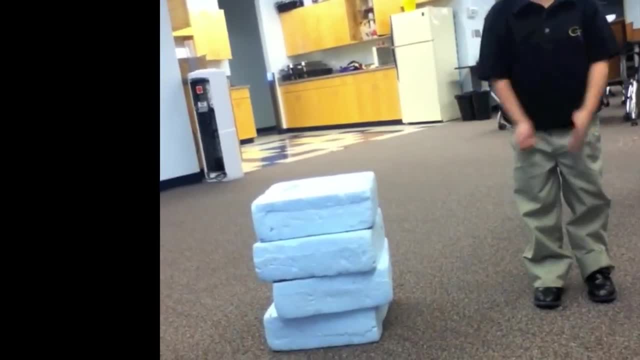 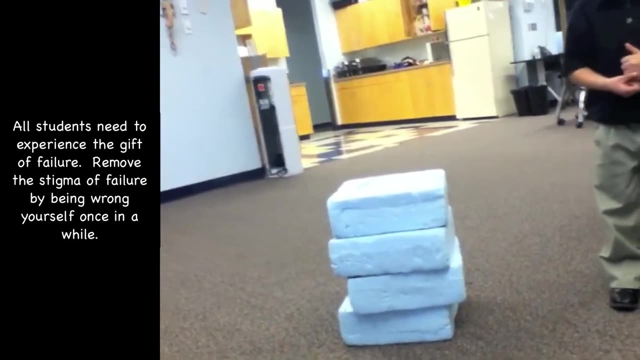 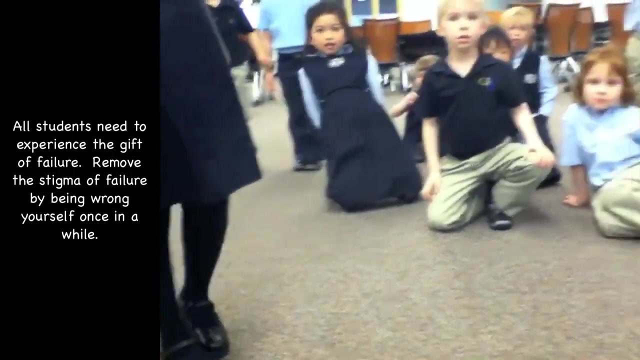 Oh, it's the same height as this one. Ah, Nope, Four, Four. Four here and five here. They look the same height, Aren't they the same height? There's four here and five there. Oh, ah, there are five there. 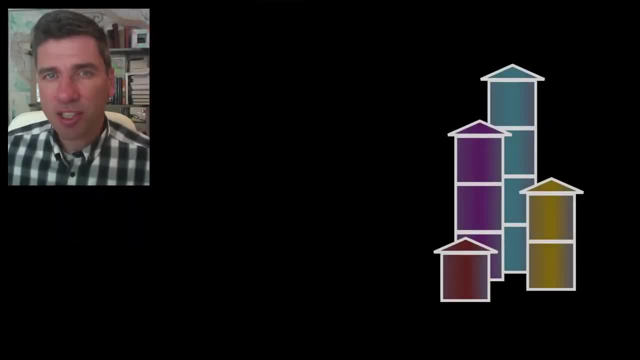 Yeah, you're right. The fairy tale king doesn't only want to know one solution to his problem, He wants to know all of the solutions to his problem. That's going to give your students a headache. They're going to have to get organized. 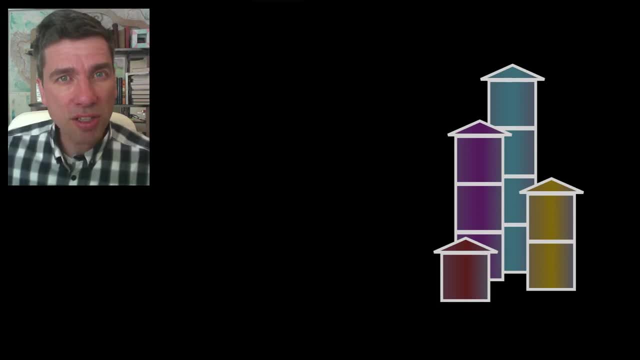 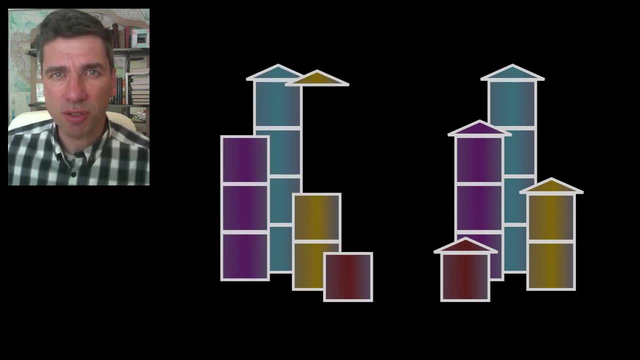 They're going to have to get organized to find all of those solutions. They might also come up with some nice questions. For example, they might ask: is this a different solution or is it the same solution? Well, you'll have to ask the fairy king- and I'll leave that up to you- what your answer. 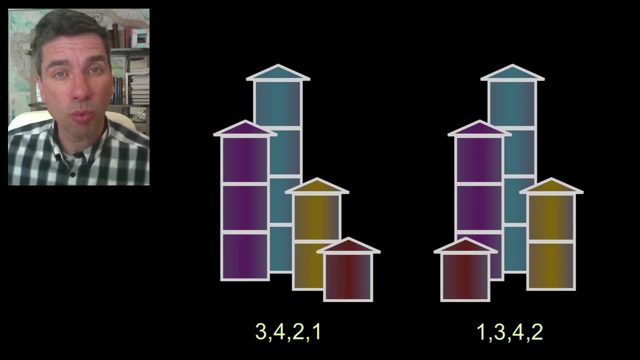 is. If you decide that 3,, 4,, 2, 1 is a different answer to 1,, 3,, 4, 2, well then you're in for a lot of solutions to the puzzle. So you might decide that that is that those two are actually the same. 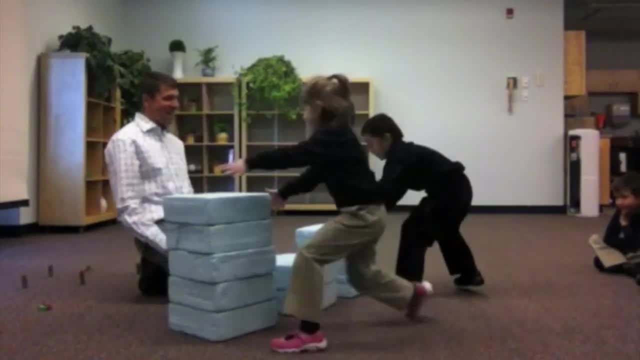 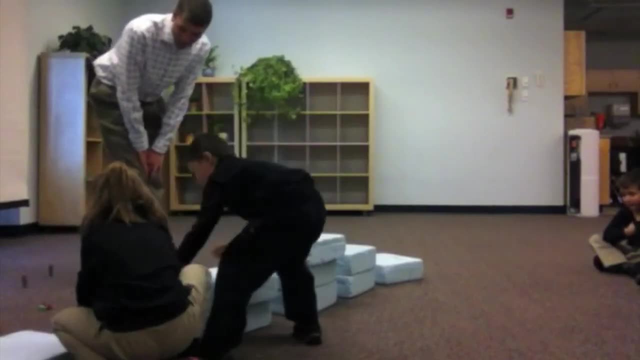 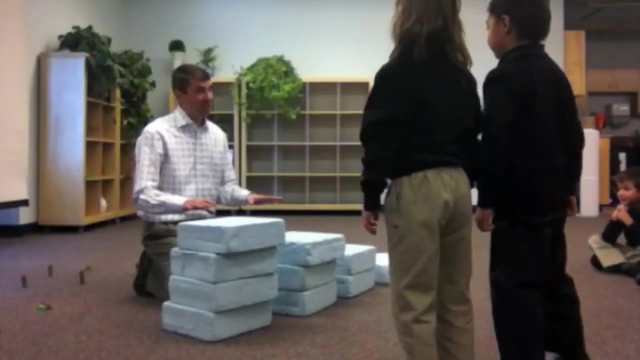 Are you ready? Yeah, Get set. Go 10,, 9,, 8,, 7,, 6,, 5,, 4,, 3,, 2, 1.. Okay, 0.. Do you think you've been successful? 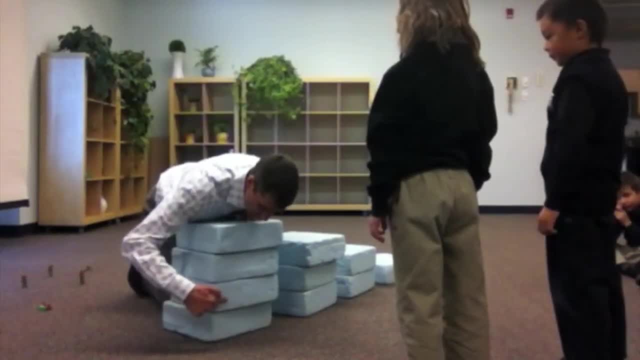 Yes, Okay, let's see: 1,, 2,, 3, 4.. 1, 2,, 3, 4.. 1, 2,, 3, 4.. 1, 2, 1.. 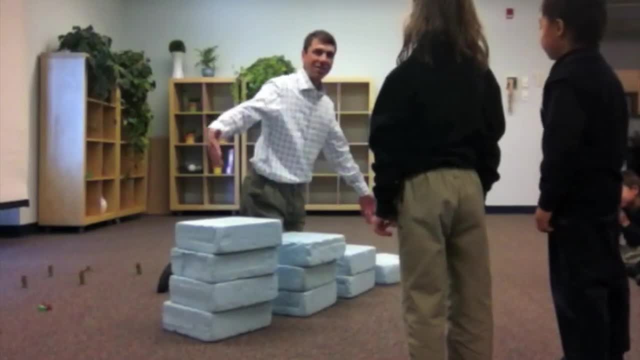 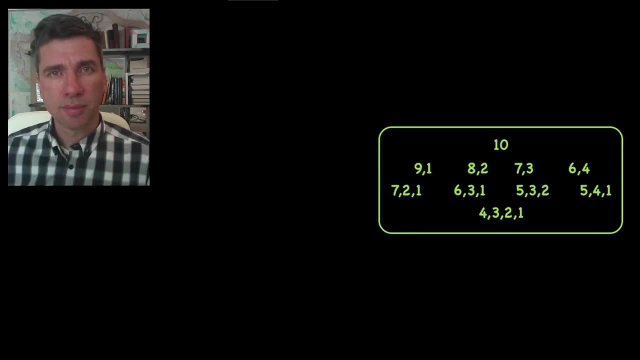 Okay, this is kind of like a staircase of buildings that you've designed. Did it work? Yes, Yes, it worked. They're all at different heights. Let's look at two ways that children have organized their results. In this case, we're not considering that 7, 3, 1 is different from 7, 1, 3.. 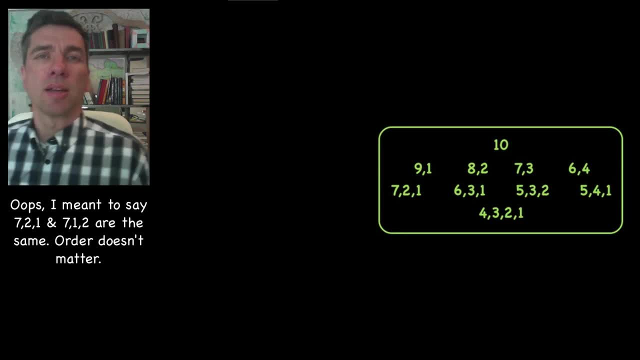 So order doesn't matter. Okay, So here, the way that it's being organized, The students have put at the very top the single solution that just has one tower. Under that they've put all of the solutions that have two towers, all of the solutions. 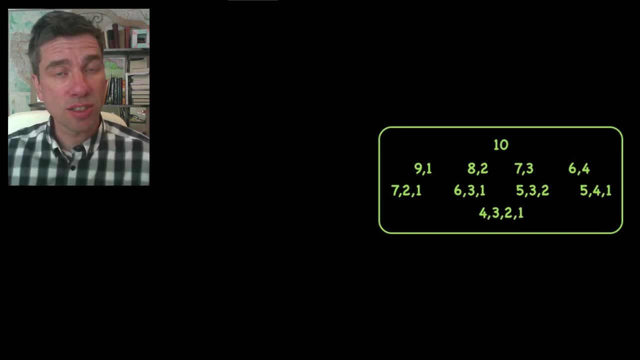 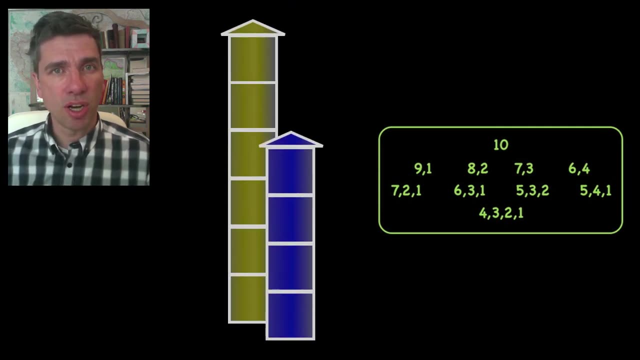 that have three towers and lastly, at the bottom, the single solution that has four towers. So, for example, this is 6, 4, and it belongs in the second row because there's only two towers. Another way that students organized was binary. 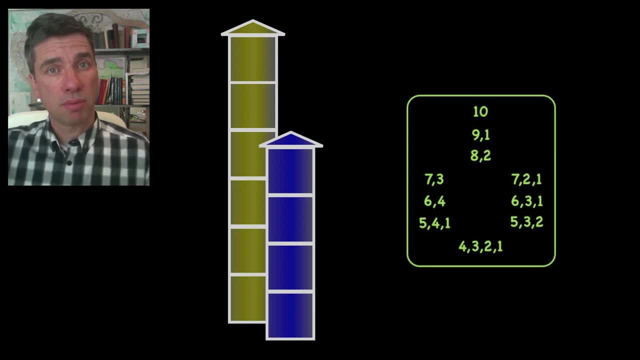 Okay, By the highest tower. So in the top they put the single tower of height 10.. Next they put the single solution with a tower of height 9, then single solution with a tower of height 8, then the two solutions with a tower of height 7, the two solutions. 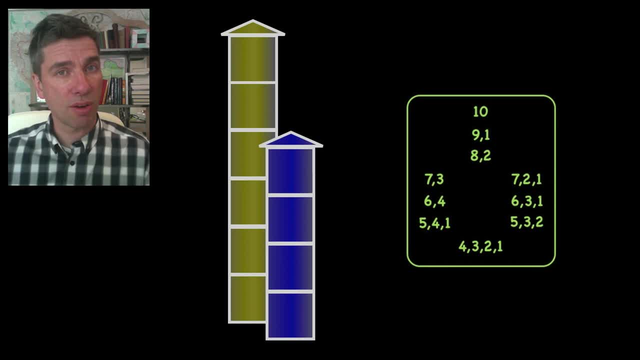 with a tower of height 6, the two solutions with a tower of height 5 as the highest, and then the single solution with a tower of height 4 as the highest. This is a rich activity, activity to get your students organized about mathematics. 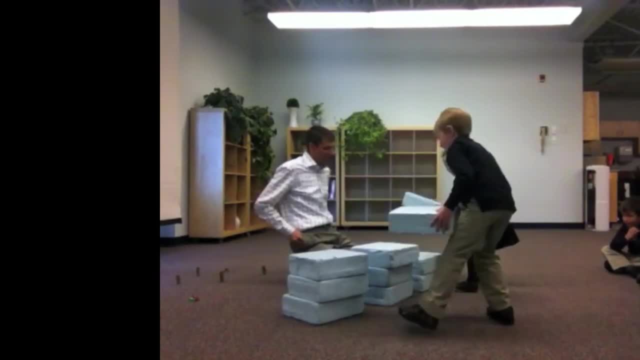 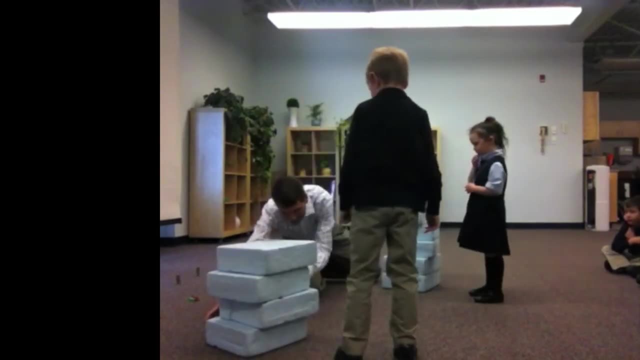 Okay, come on. 10,, 9,, 8,, 7,, 6,, 5,, 4,, 3,, 2,, 1, 0.. Okay, What do you think? Did it work? No? 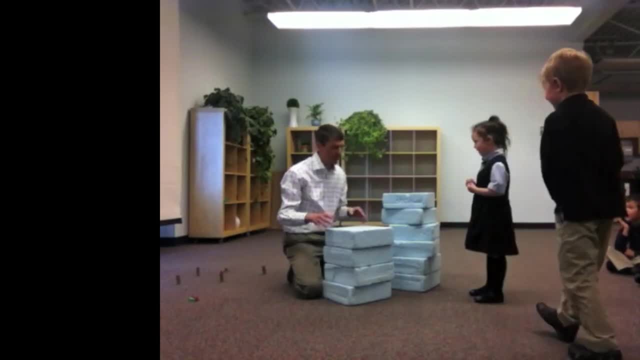 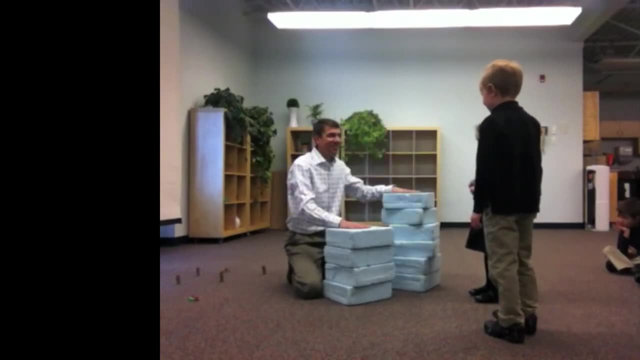 Are they at different heights? Some of them are 1,, 2, 3, 4.. 1,, 2,, 3,, 4,, 5, 6.. Yes, That's acceptable, But have you seen this solution before?